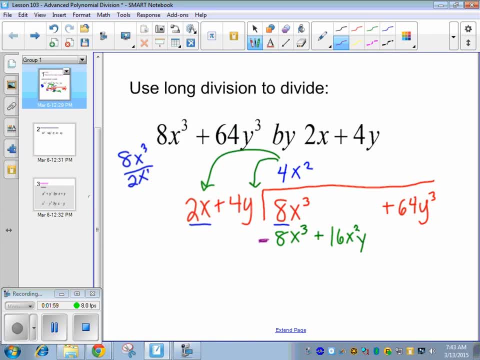 Change. Change the signs. So we subtract this and then this one's going to change also to subtraction, So you change both signs. These cancel and they should. And now I have negative 16x squared y. Normally we bring down the next term, but I don't want you guys to do that yet. 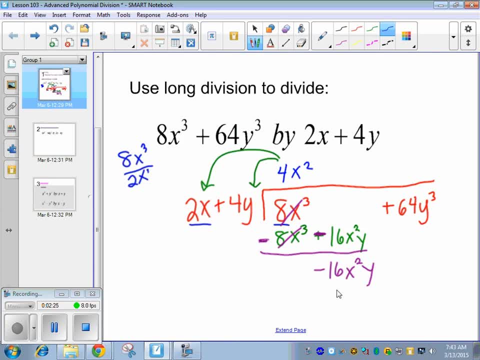 Okay, So we just do. we start over this first term here, Divided by just this first term here. So negative 16, I'm going to write that up here so I can see what I'm doing: Negative 16x squared y, and we're dividing by just the first term, 2x. 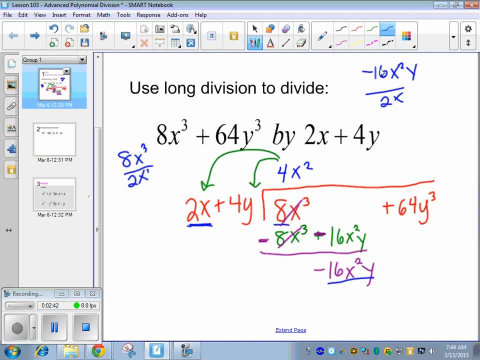 What do we get for that? Yep? negative 8, and then we get a 1x and we still have this y here. So negative 8xy Y. After you put this up top, you multiply, You multiply it back through and it multiplies to both terms in the front. 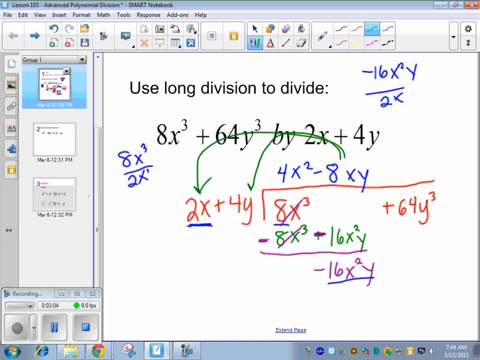 So negative xy is going to multiply by this and negative xy is going to multiply by this. So negative xy times 2x. What does that give me? Thanks, Negative 16x squared y. We should get exactly what we have there. 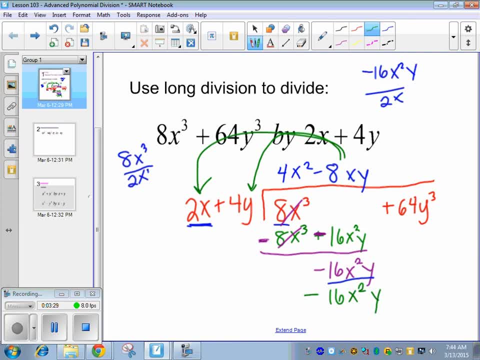 Right, And we are multiplying a negative by a positive. So negative 16x squared y. Now we have to multiply it by the 4y, right here. So don't forget to do this. This is the biggest mistake I see is that people don't multiply this times. this. 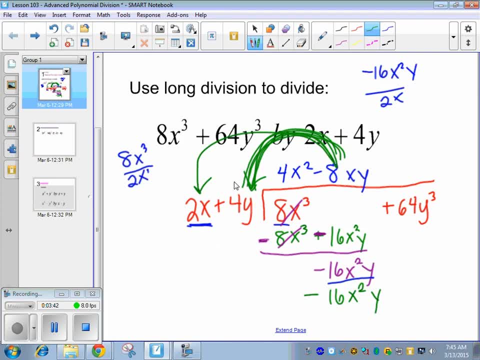 So now what do I get when I multiply these together? What's 4 times 8?? Okay, 32.. Then we have an x. What's y times y? Okay, So negative 32.. So we have 32xy squared. 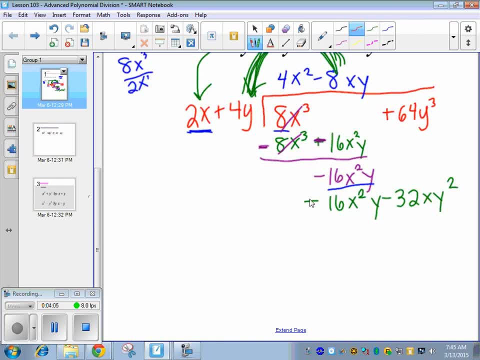 What's the next step? Change the sign. So I'm going to add, and I'm going to add These: cancel out and we have 32xy squared Leftover. And now I'm going to divide the first thing by the first thing. 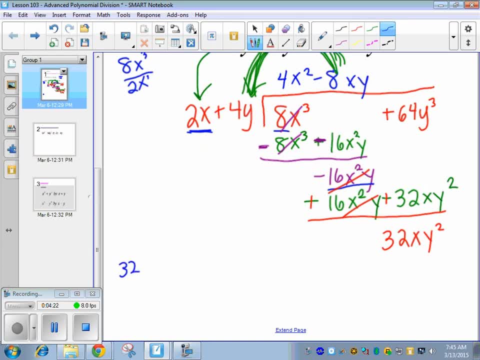 So these two terms. So off to the side. I have 32xy squared and we're dividing by 2x. What's 32 divided by 2? 16.. The x's cancel out and we still have y squared. 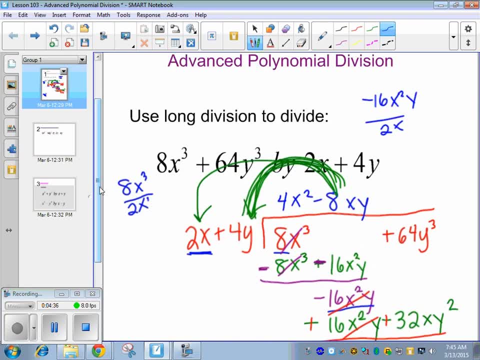 All right. So 32 divided by 2 is 16, and then I have y squared. We write that up top. So plus 16y squared. After we write it up top, we multiply it back through times, both terms. Okay, times, both terms up here. 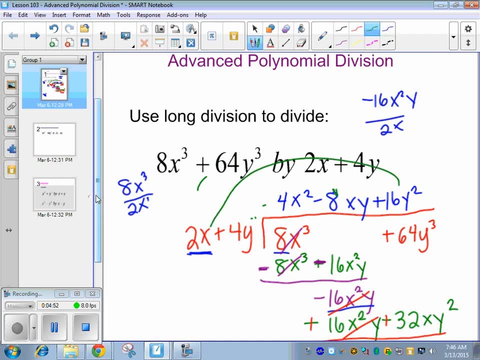 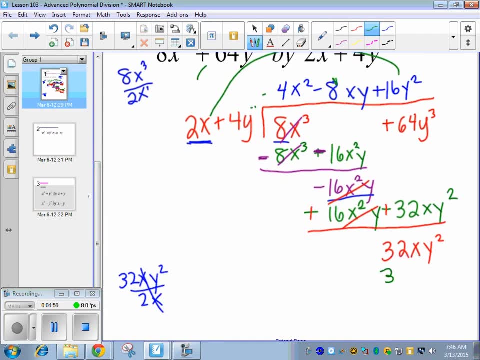 So what's 16y squared times 2x 32, and then we have an x and a y squared- It should match this right. And then we have to multiply it times the second term, right here. So what's 16 times 4?? 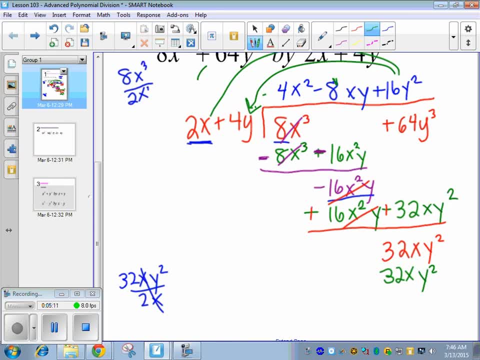 64.. What's y squared times? y y cubed? All right, once this matches this, you can go ahead and bring that one down, Okay, Okay, because we're going to now subtract, So I'm bringing down what was finally my last term. 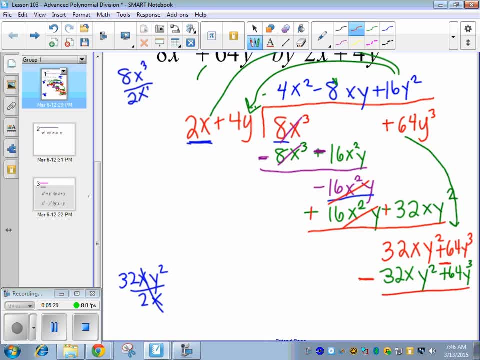 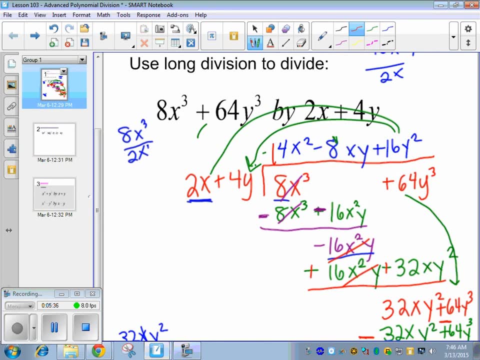 and our next step is to change the signs and it goes in evenly and we get 0, which means we have a final answer of 4x squared minus 8xy plus 16y squared. Okay, Let's try another one. 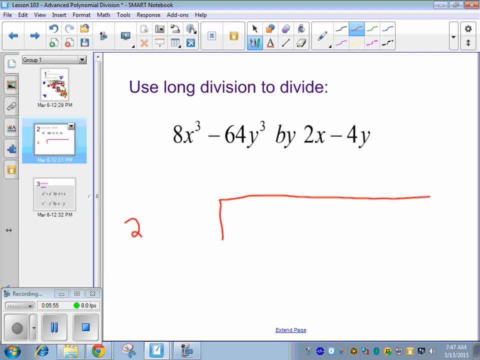 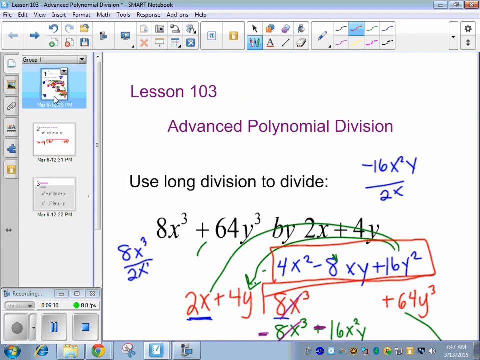 All right. so 2x minus 4y goes on the outside, 8x cubed minus 64y cubed goes here. So it looks very similar to the last one, except for last time we had positives, Now we have some negatives. 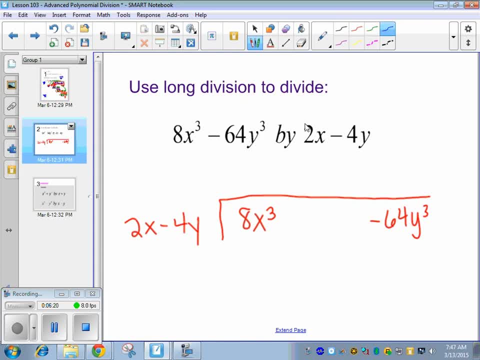 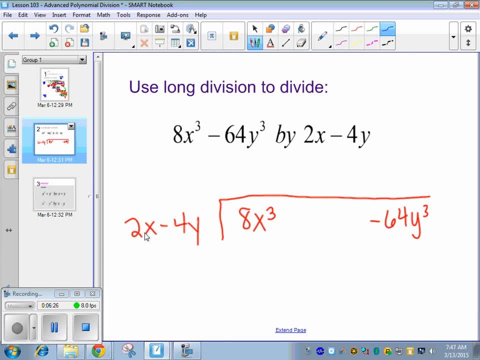 Multiply 8x cubed times 3y, Not multiply, Not multiply. Add, Not add. Divide, Divide, Okay, 8x cubed divided by 2x. So, Kevin, what is that? 4x squared? 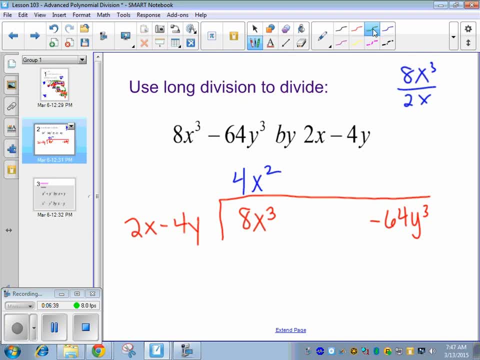 All right, so we put 4x squared up top, Devin. what do I do next? after I put a number up top, Multiply it by 2y. Okay, good. So, Patrick, what do I get when I multiply this times this? 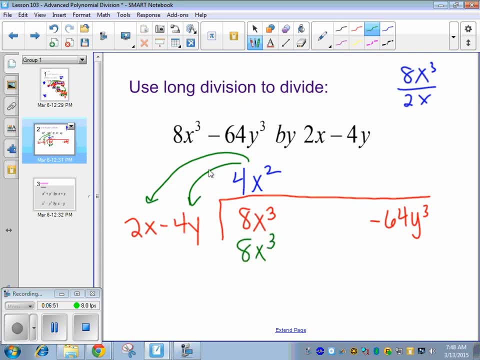 8x cubed, 8x cubed And Patrick. what do I get when I multiply this times this? What's this Negative? 16x squared y Nice, Okay, All right, now we start over and we divide this by this. 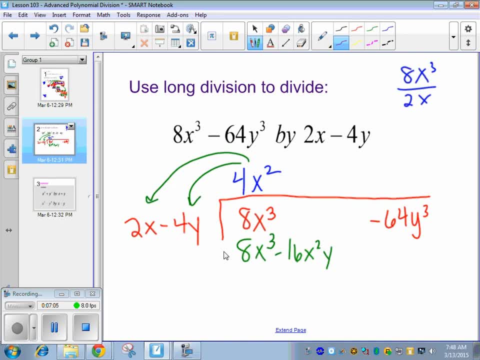 The first by the first? Actually, no. Before we do that, what do we do? Change signs. My bad, Sorry. All right, change signs. This cancels. Add down: We get 16x squared y. Now we divide. 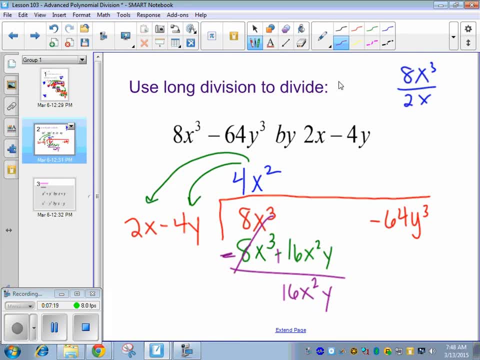 So, Grace, what do I get when I divide 16x squared y by 2x 8x squared y- Okay, 8xy Good Plus 8xy Okay And Payton. after I write anything up on the top, what's my next step? 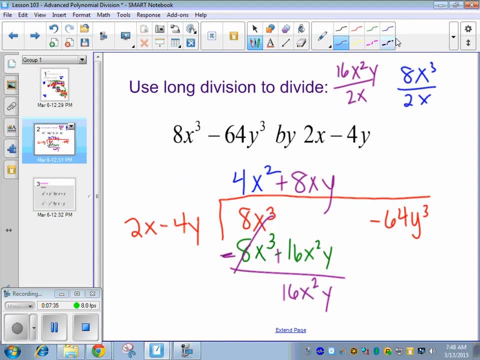 Yep, Multiply it back through times both terms. So, Zach, what do I get when I multiply 8xy times 2x, 16x squared y? Okay, We should get the same thing. And, Max, what do I get when I multiply 8xy times negative 4y? 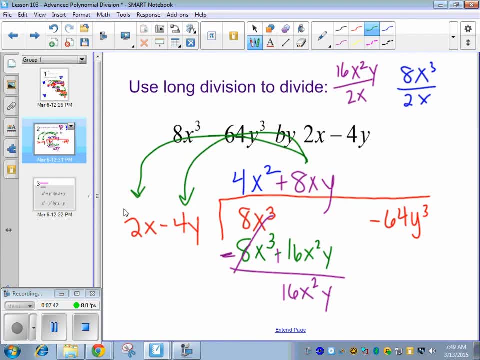 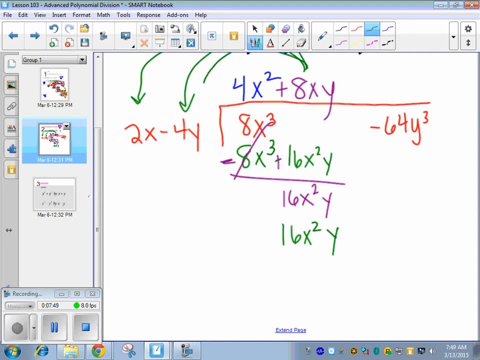 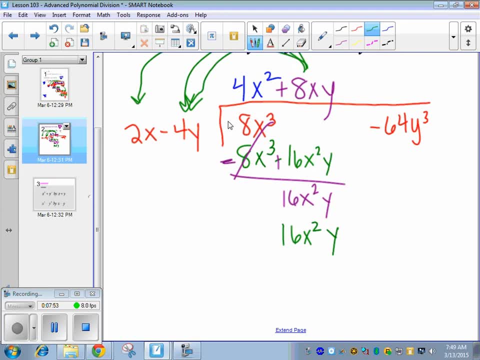 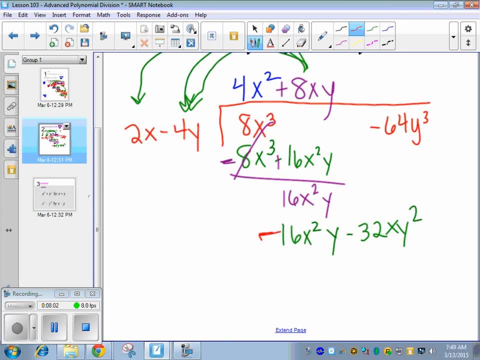 Negative 32xy squared. Very good, All right. And Isabella, what's the next step? Yes, Change the signs Minus and plus, So those cancel. We now have a plus 32xy squared. Okay, Abby, what's the next step? 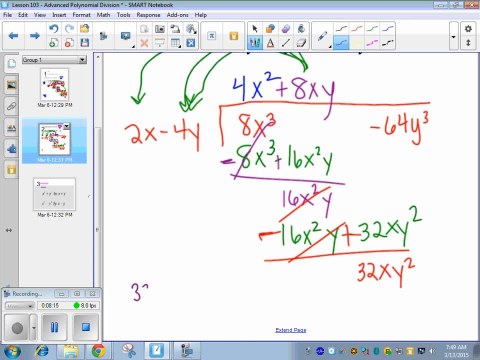 Divide 32xy squared by 2x, Yep, Divide 32xy squared by 2x, And Cole, what do I get? 16 y squared. Okay, and after I write anything up top, Connor, what's the next step? 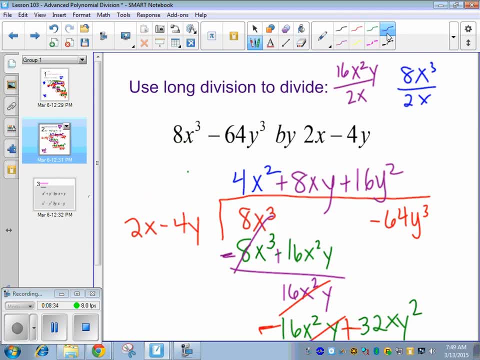 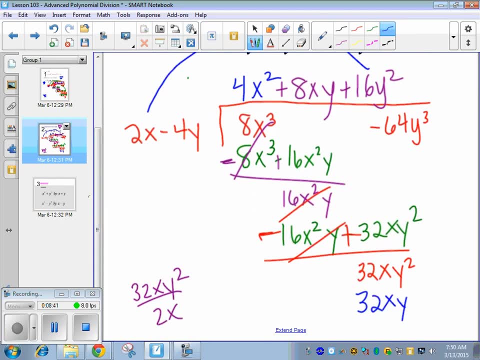 Multiply that by both of them. Okay, multiply it back through, Alex. what do I get when I multiply 16 y squared times 2x, 32 x squared Good And Natalie. what do I get when I multiply this times this?